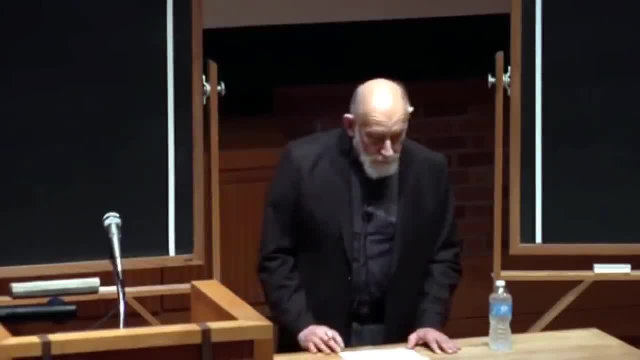 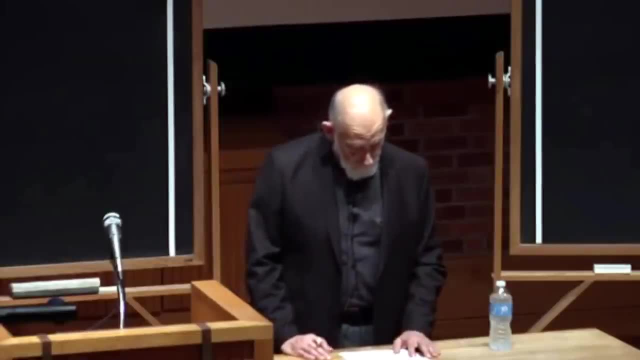 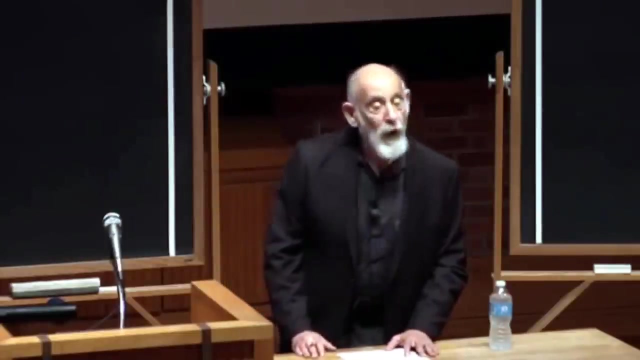 It's generally deemed that Bohr won the debate, but in retrospect it's clear to me that Einstein's view was by far the deeper. Bohr, I think, never really understood entanglement. In essence, he told Einstein: go home and take an aspirin. You'll feel better in the morning. Einstein. 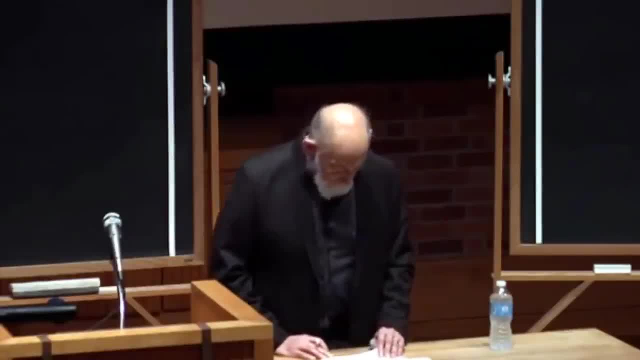 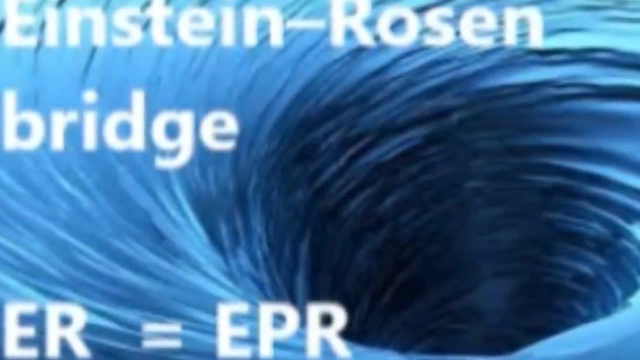 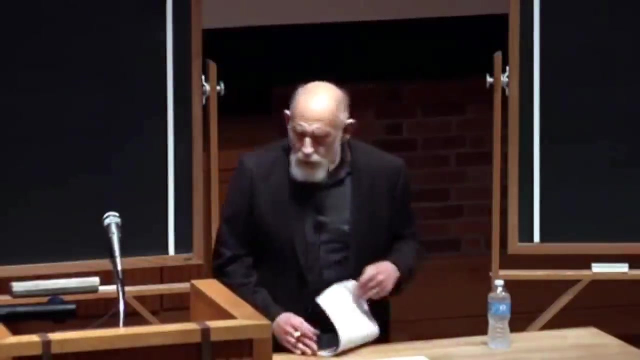 didn't want to feel better. He wanted to understand it. In 1935, long after, incidentally, he was considered to be irrelevant- Einstein wrote two papers on two entirely different subjects. At the time they were widely dismissed. The two papers will be known. Can this be? 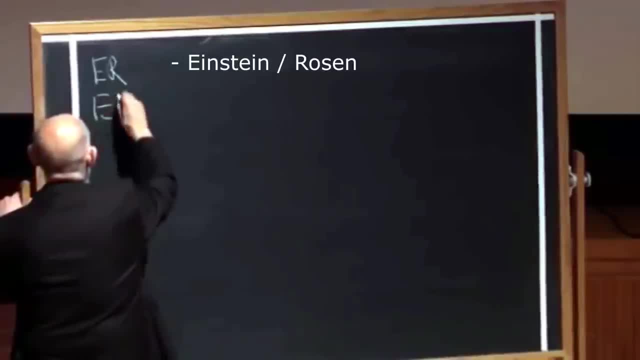 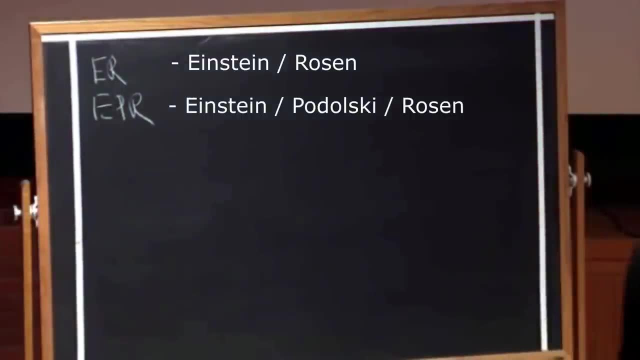 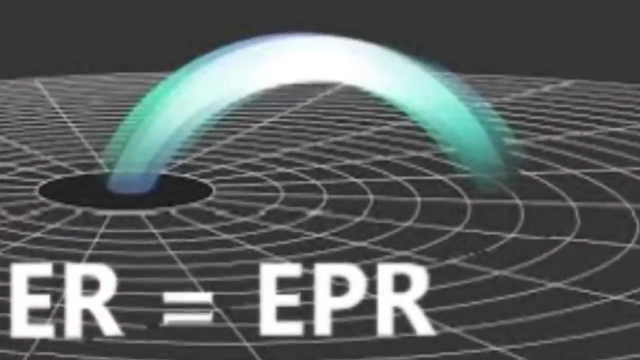 seen EPR. ER stands for Einstein and Rosen. He wrote the paper with Nathan Rosen. I will tell you what it was all about as we go along. And EPR stands for Einstein-Podolsky and Rosen. As I said, these two papers were on entirely different subjects As far as 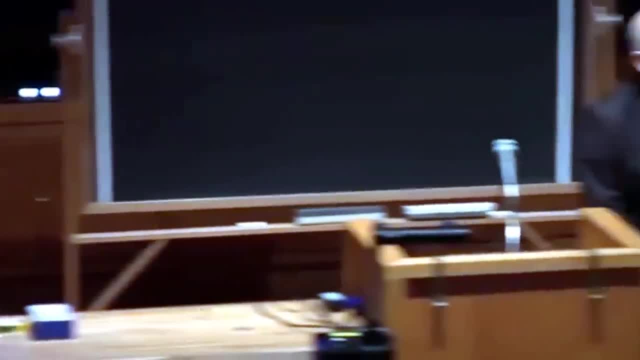 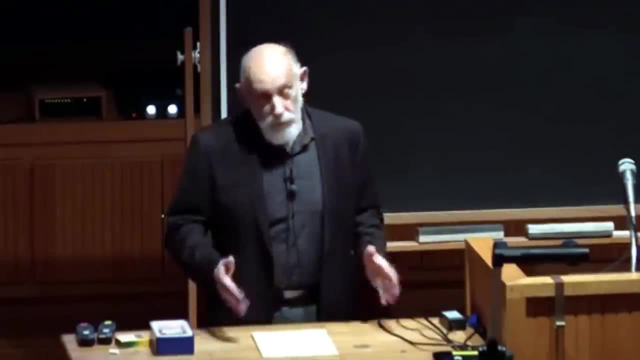 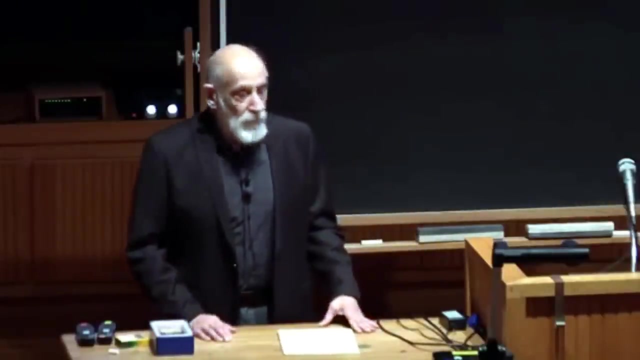 I know neither Einstein nor anybody else had any reason to believe they were connected. In classical physics you can know the exact state of a system. Sorry, you can always know the exact state of a system. Knowing the exact state of a system in classical physics entails: 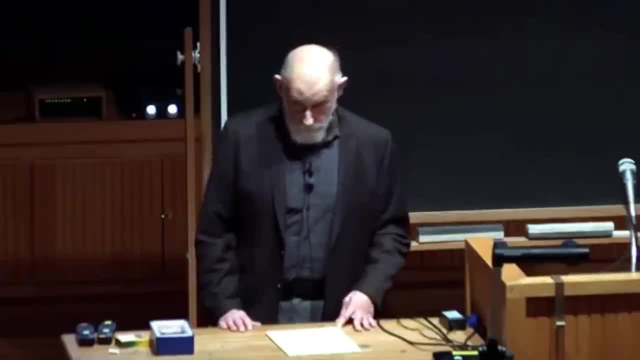 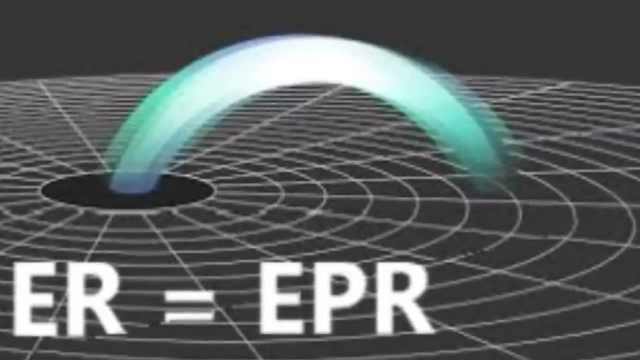 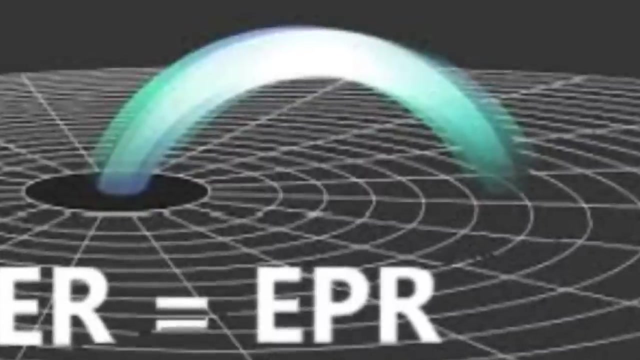 knowing exactly what's going on with each of its parts, But in principle, without disturbing the system significantly, we could have known more about it than we did. All right, Let's begin with EPR. EPR, Einstein, Podolsky and Rosen. It also happens to stand. 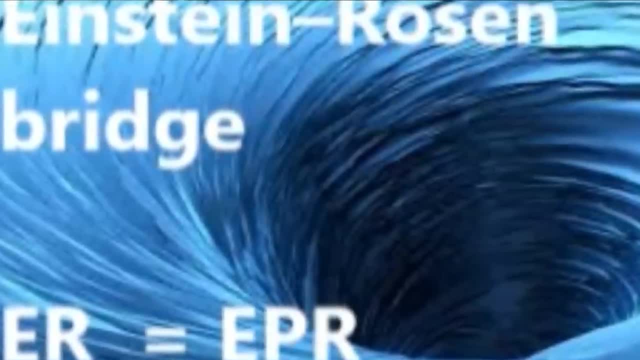 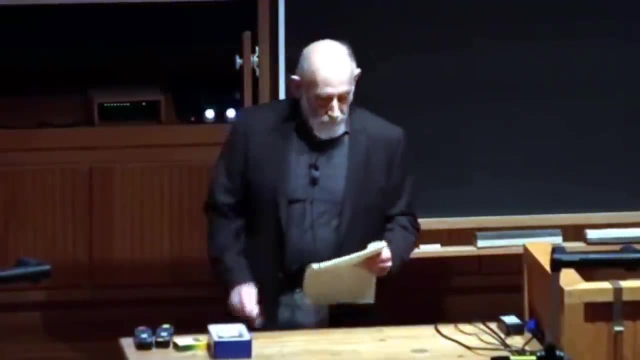 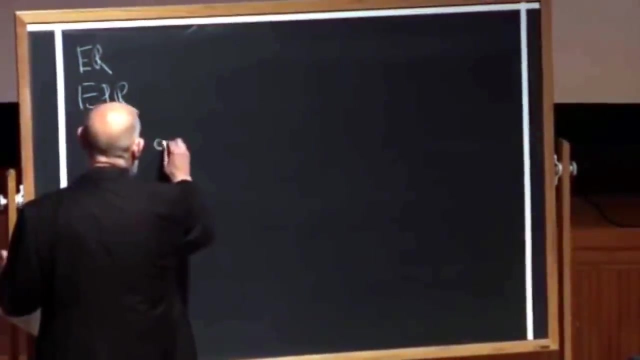 for a term that they used in their paper: elements of physical reality. This was something that disturbed Einstein a lot, but let me give you a very, very quick quantum mechanics lesson. Here it goes: We have A spin. A spin is a little physical system. For the moment let's not even worry about 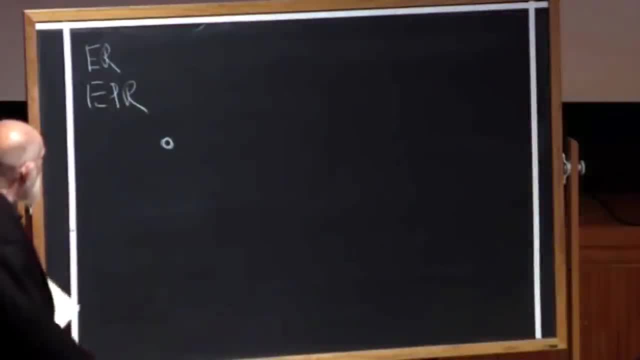 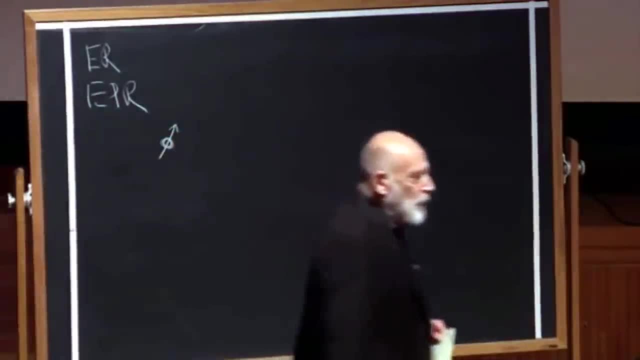 what it's attached to. In practice, it would be attached to an electron, but it's a little system and it has an arrow associated with it, In other words, a vector. It's something you can measure and when you measure it, you measure its components. It's X component. 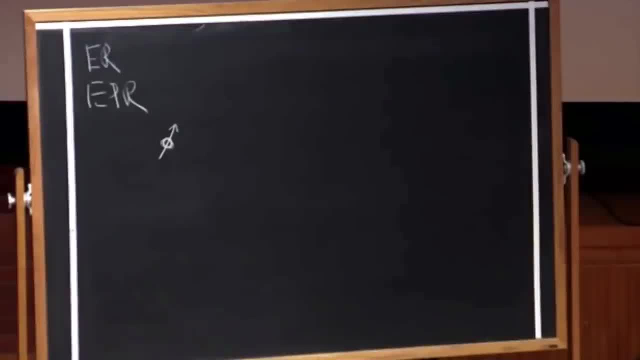 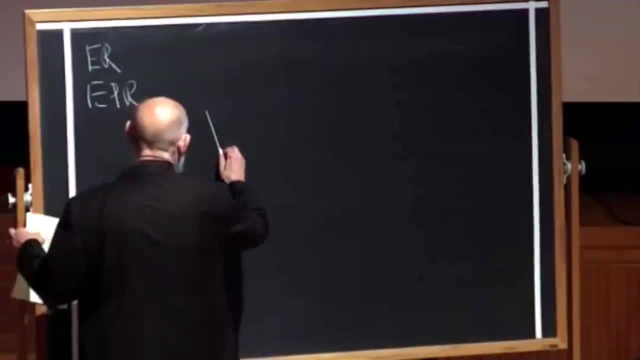 it's Y component and a Z component, and so forth. So let's add another system. The next system is the apparatus that we use to measure it, And the apparatus looks like this: It's a box, It's a black box. Well, it's not black. 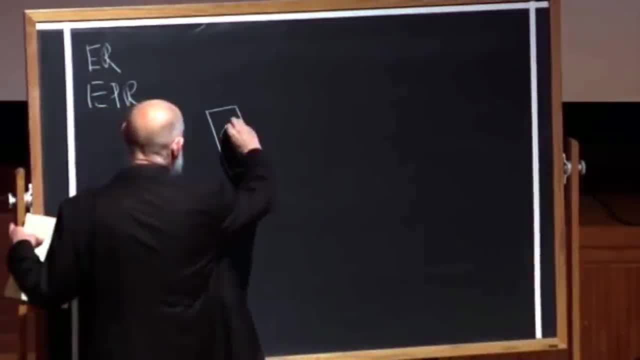 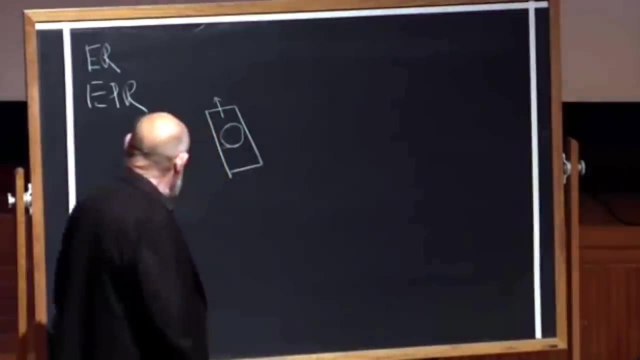 It's just a box. It has a little screen on it that will show an answer. It has an arrow on it that says this way up in order to tell which way it's oriented, And you can orient it in any direction in three-dimensional space that you want. It also has a button here. 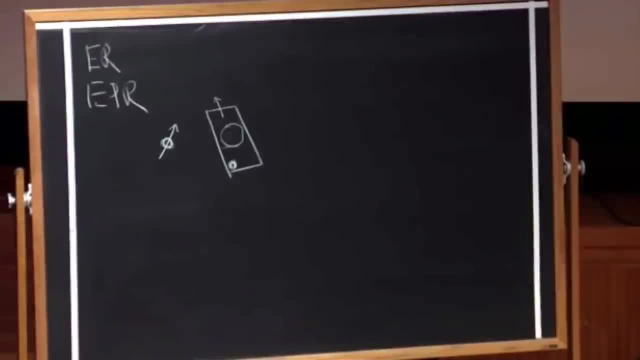 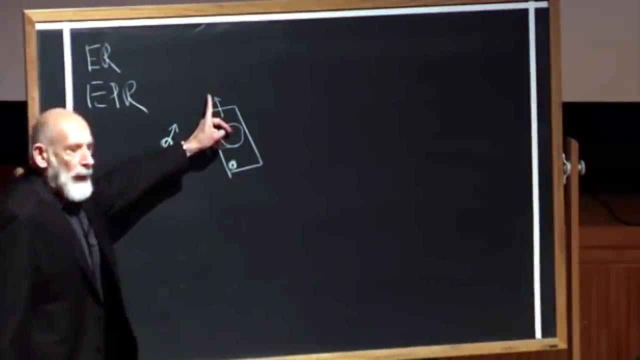 The button says M for measure. You bring the apparatus up to the spin so that it's in contact with it. You press the button and you get an answer. Purportedly, the answer is supposed to be the component of the spin along the axis of the detector. You will always get in quantum mechanics. 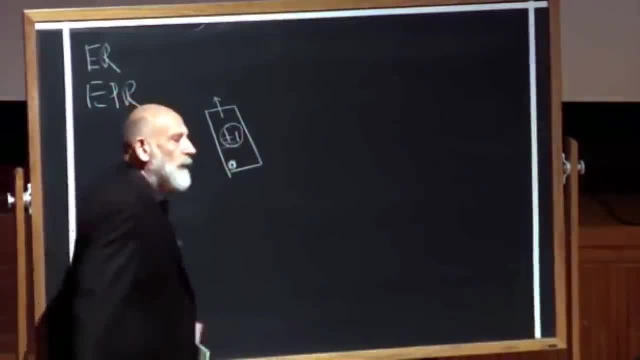 either plus or minus one. No intermediate answer, nothing in between: either plus or minus one. This is a little bit peculiar, that the component of a vector in an arbitrary direction should be plus or minus one. but we understand this. This is quantum mechanics. This is the weirdness of quantum mechanics, but it's OK, We did. 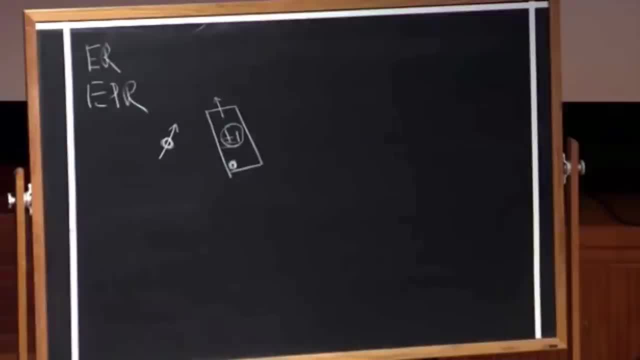 our homework, and that's a consistent thing to happen. Now, it is also true that for any state of the spin, in other words, for any precise way that you set up the spin, any state, which means any specification, complete specification. 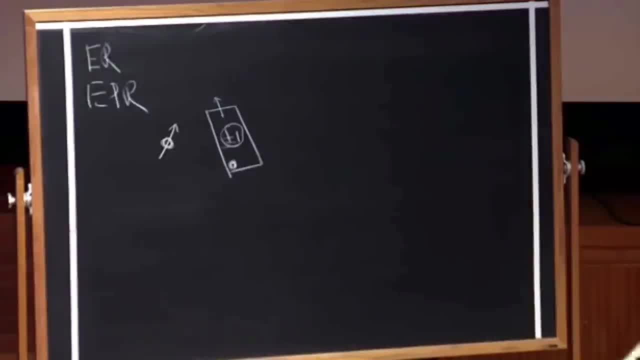 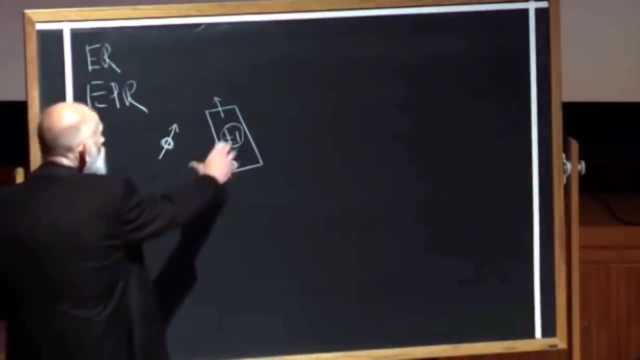 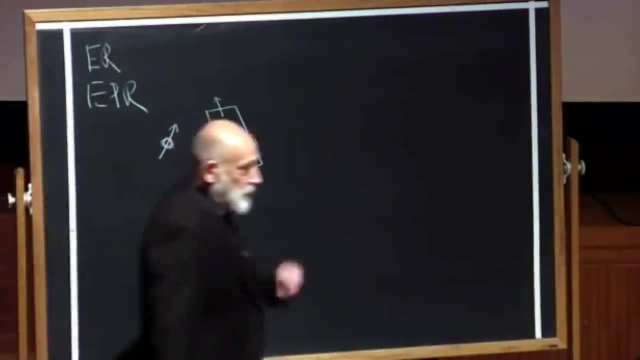 of everything that you can know about the spin, everything that you can know that there is always a direction that's called a polarization direction, that if you oriented the apparatus in that particular direction, you would always get plus one. In other words, there's some. 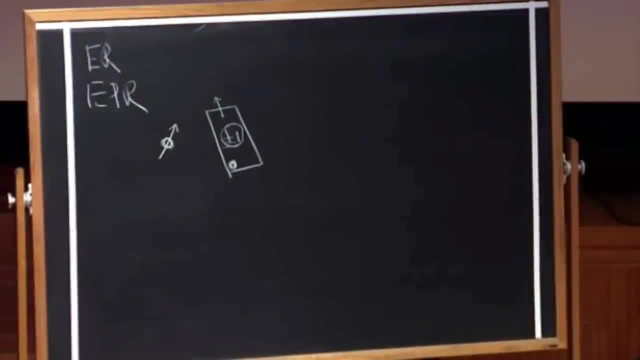 direction that we would say the spin is pointing along, that if you measure it along that direction you'll always get plus one apparatus in another direction. you'll get statistically somewhat random results. The more orthogonal the detector is to the polarization axis, the more random it is. 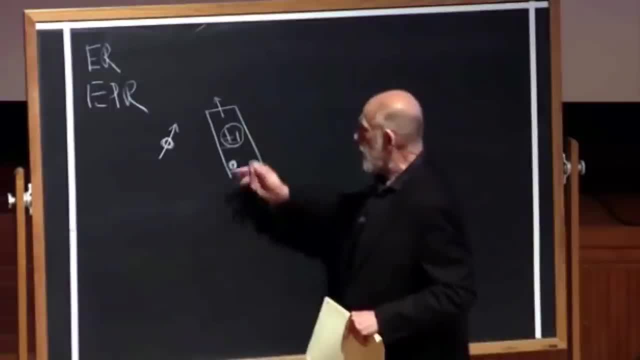 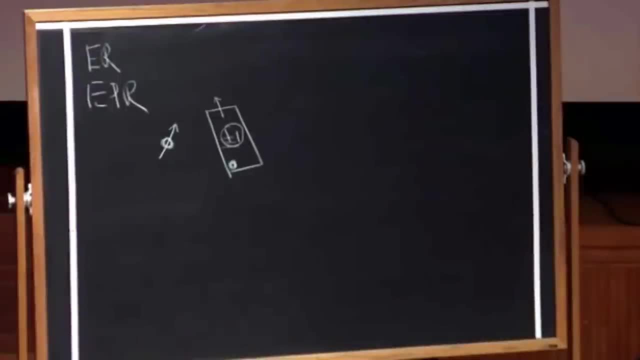 And in particular, if this arrow here lies in the plane perpendicular to the polarization of the spin, you simply get random answers. That's quantum mechanics of a single spin in a nutshell. Now next question: Can you simulate, can you fool somebody into thinking they're seeing quantum mechanics? 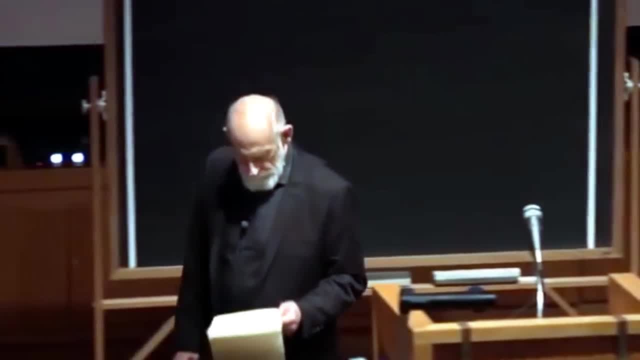 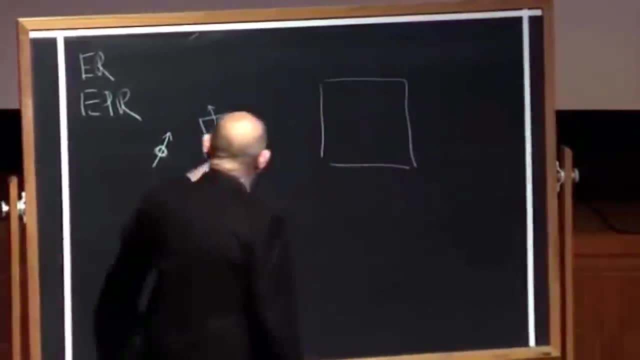 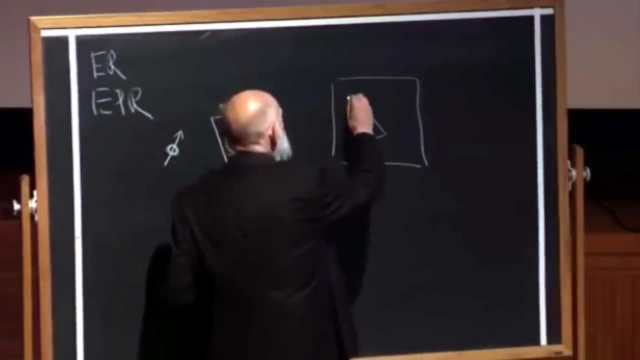 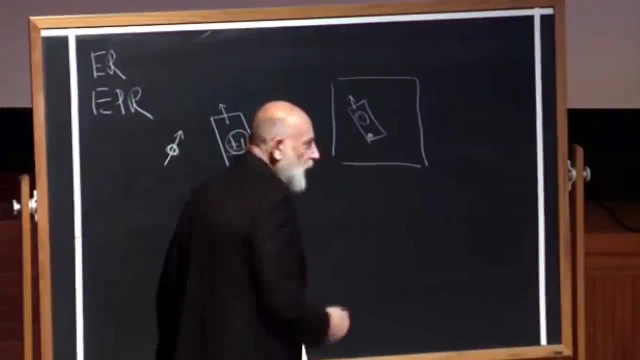 Here's your task. You have a computer. Here's your computer. On your computer screen you have a detector, an apparatus. That apparatus can be manipulated and it can be oriented in any direction. You have a little M over here and you take your mouse and you click on that M and in. 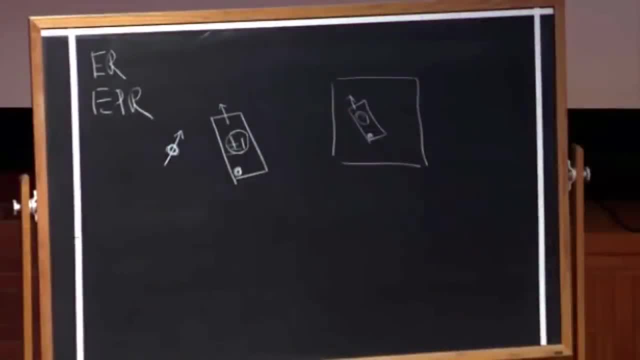 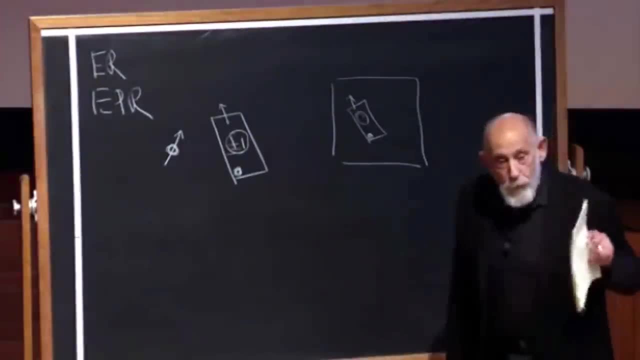 the box here or not? in the box, in a little circle, there appears a plus or minus one. The question is: can you program your computer in such a way as to fool somebody into thinking that in the computer there is a real electron? and this is measuring the real electron, and 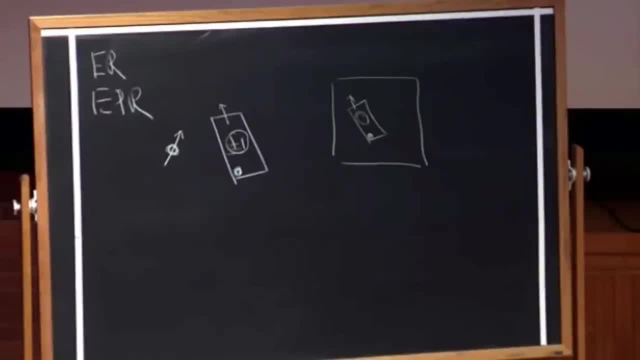 recording the result. Yes, it's not very hard. Okay, Two things, at least two things. computer scientists might figure out some more stuff that you actually need, but one thing you need is a random number generator, because you have to- under certain circumstances, you have- to generate random answers. 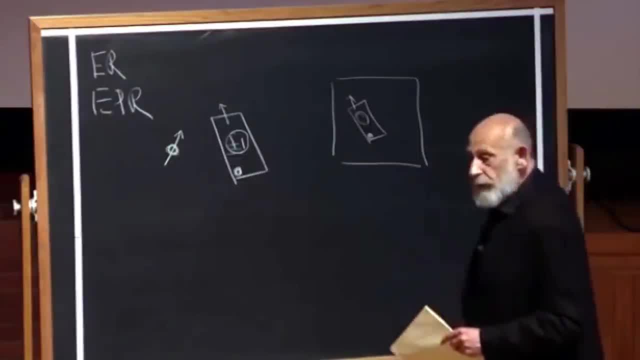 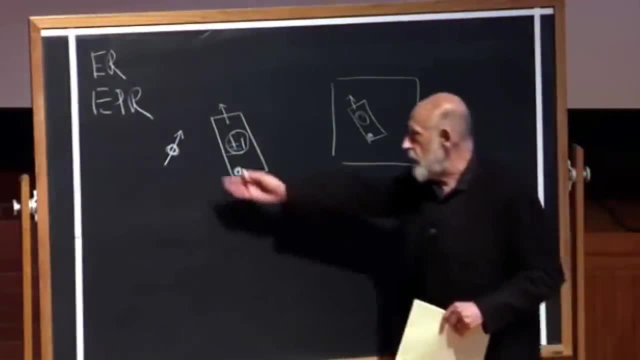 So you need a random number generator and you need a memory to record the state of the spin. Whatever the state of the spin means in this case, it simply means a polarization direction. you need to record what the state of the spin is. 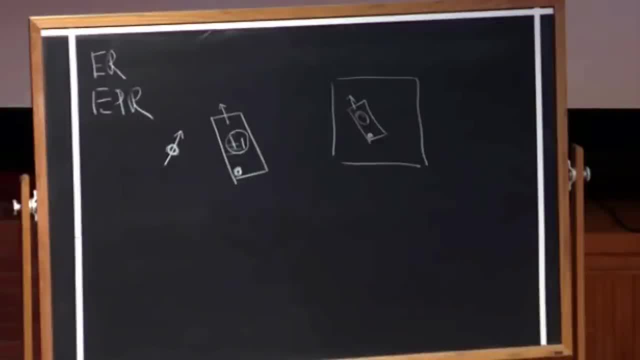 And you need to, and you need a random number generator to generate answers. That's all you need, and you can mimic quantum mechanics, At least for the single spin. Now let's come to the problem. let's suppose there are two spins. 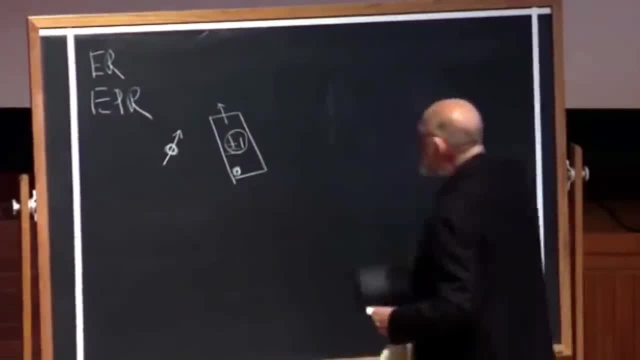 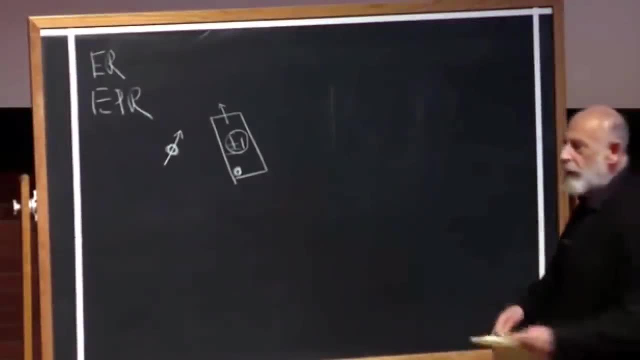 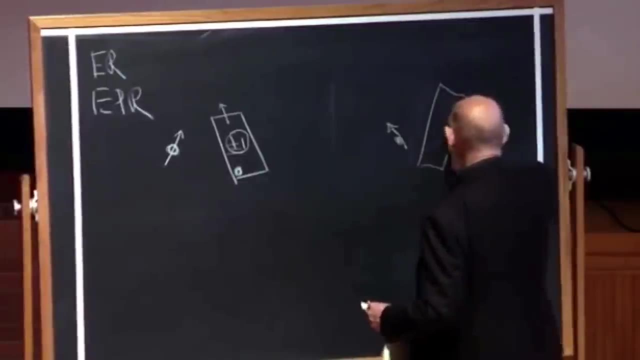 Let's suppose there are two spins And let's presume that the spins aren't Okay. They are fairly far apart so that they're not significantly interacting, they're separate. Here's another spin And here's the detector or the apparatus that's used for measuring that spin. 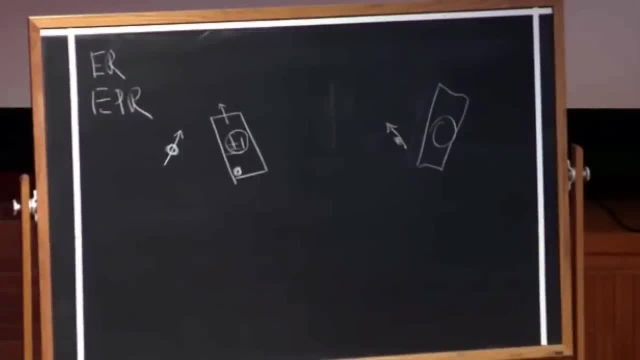 You might expect that the state of a two-spin system is simply specified by specifying two polarization vectors, Two polarization vectors, and that they're simply two systems Identical, each identical to the first, And in fact you can create electrons or spins in that kind of configuration. 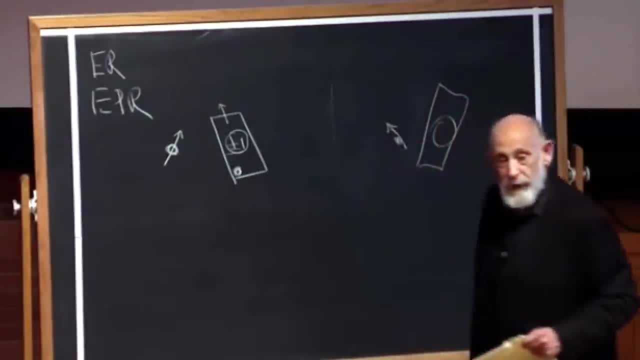 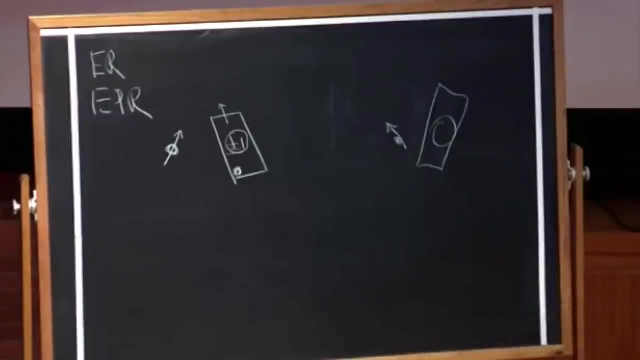 You just do it by, uh, separately and independently arranging the two states of the two spins. It's called a product state And a product state. there's not much crosstalk, no crosstalk between them, no correlation between them, not even any interaction between them. 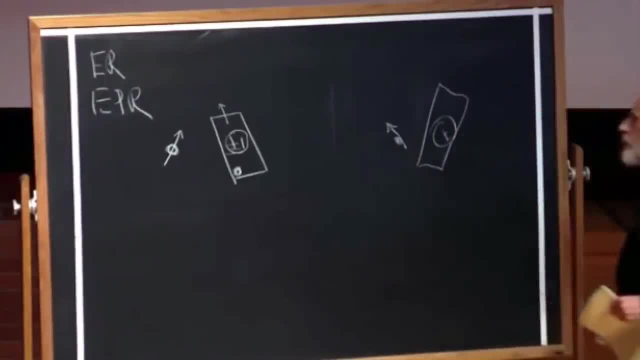 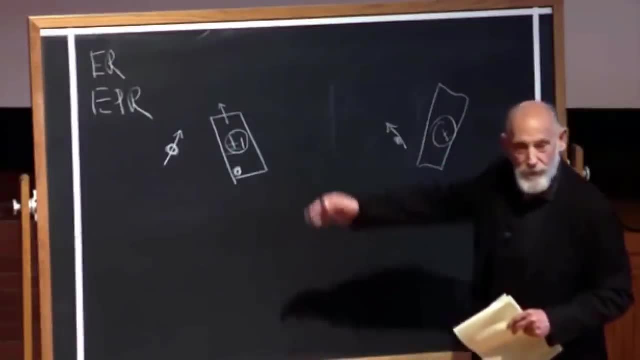 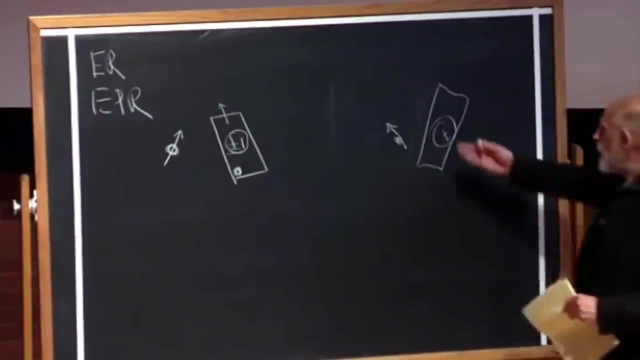 And the two sets of experiments are completely independent. each apparatus has its own random number. well, this is for the real spins. question is: can you simulate this? of course you can simulate this. to simulate it, you simply have two random number generators, two memories, one over here, one over here. 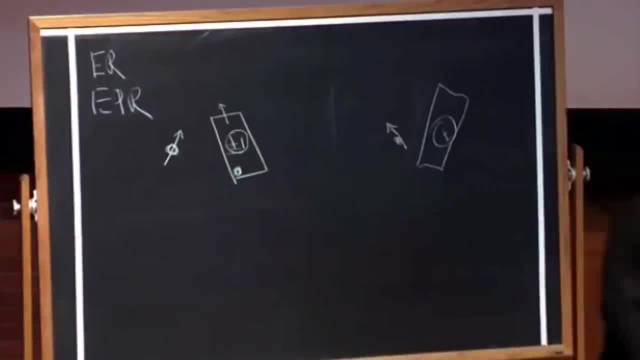 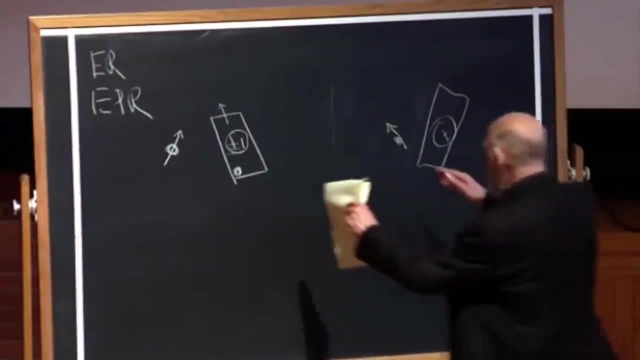 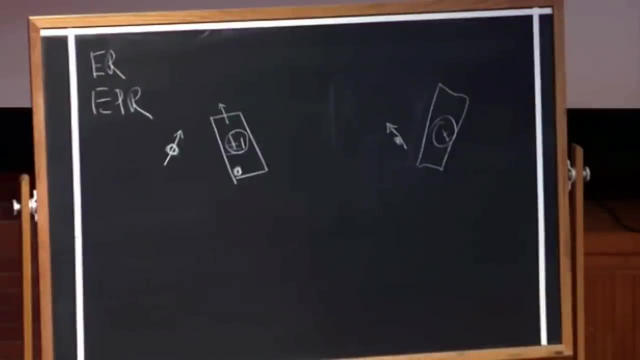 and you just do in each place the same thing that you would have done with only one spin. so, yes, you can simulate that. but there are a wider class of states available to two spins and the additional states are called entangled states. for those who know quantum mechanics, I will write down an example of entangled states. 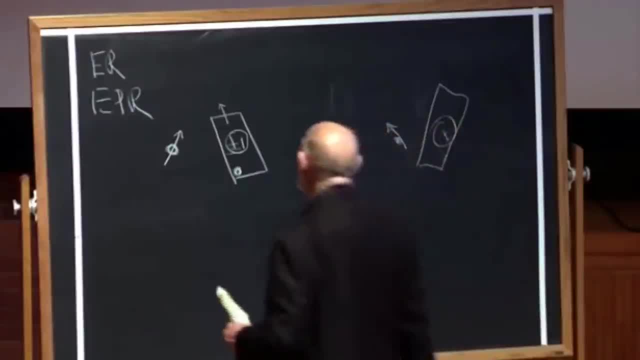 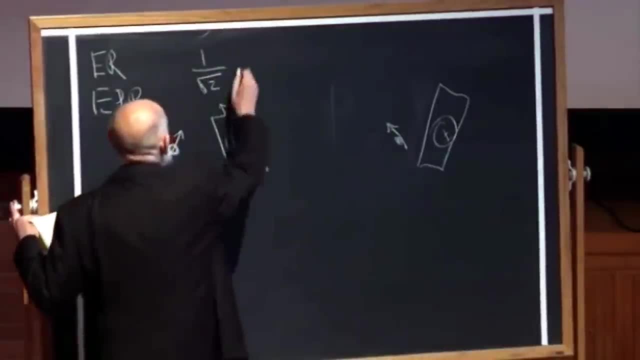 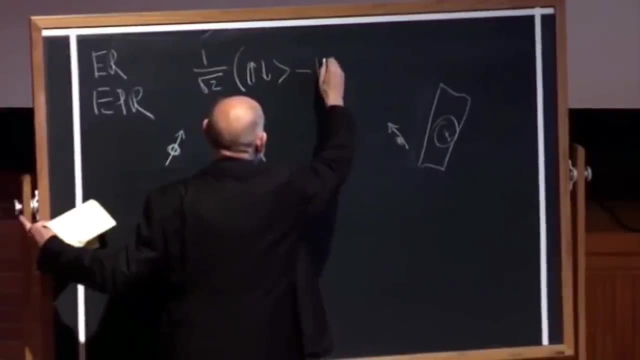 and I will never use it again. but I will not explain it, I will just write it: one over the square root of two times a state in which the first spin is up, the second one is down, minus the first one down, the second one up. this is a quantum mechanical combination. 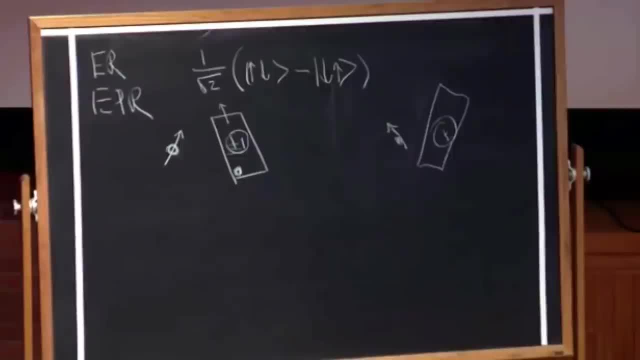 of two states, in which one of the states has one spin up and the other one down, and vice versa and vice versa. this is a proper quantum mechanical state. it's a complete description of the system. there's no more to know. you cannot know anymore. quantum mechanics says that's right, but why so? 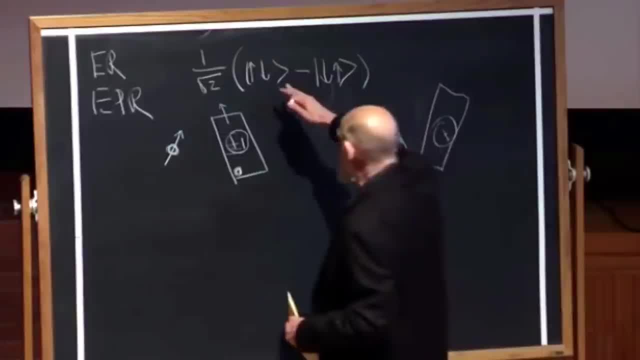 There cannot be any more knowledge once you know the state of the system, but it has some odd properties. Let me tell you what they are, The odd property that I find most interesting. Of course, there are detailed mathematical consequences of this, but I'm just going to focus on one very, very simple observation. 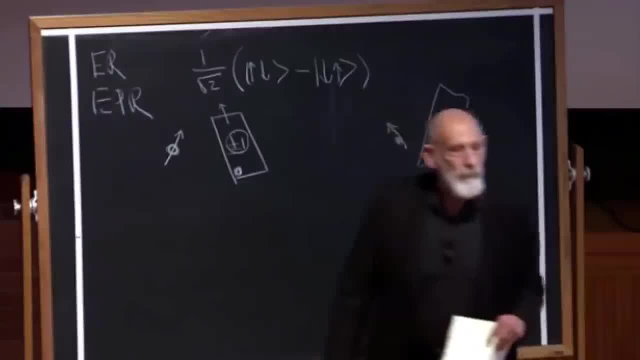 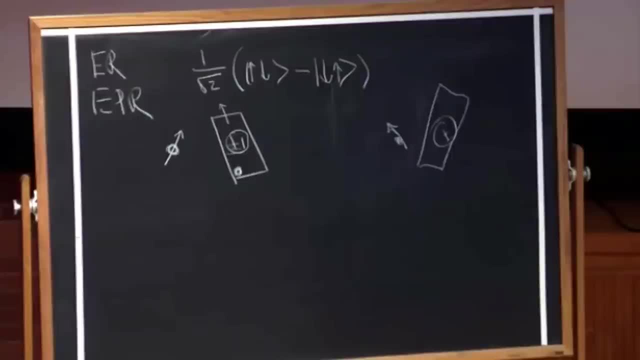 If, in this type of state, you measure either of the two spins in any direction at all, you'll get a random answer. It doesn't matter which way you tilt your apparatus, you'll always get a random answer. In other words, in this case there is no polarization vector for either of the spins. 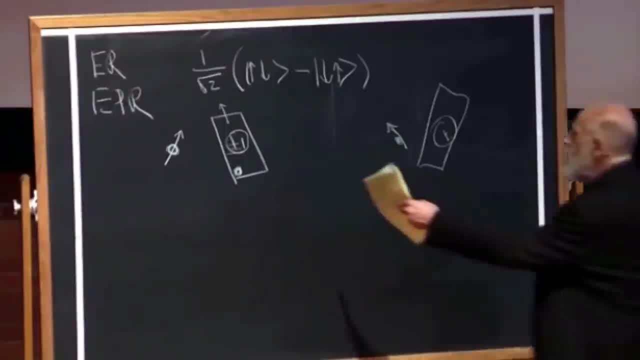 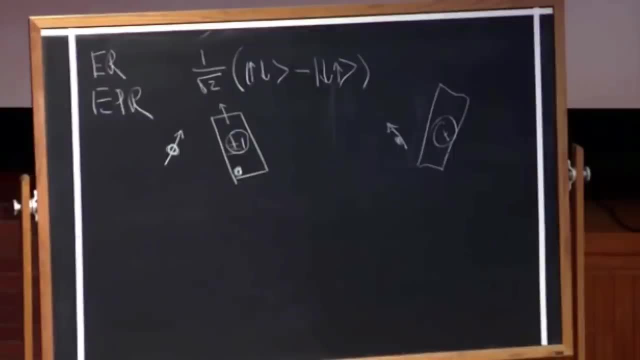 and it simply doesn't look like a state of two independent spins, Either spin or both spins. if you measure them, you will get random answers. I would say this is peculiar for the following reason: I would say that you have absolute, complete information about the composite system of two spins. 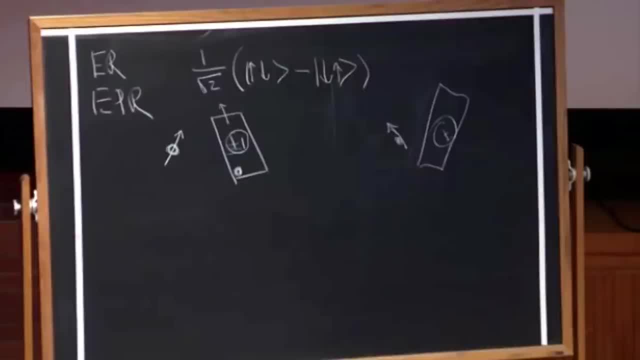 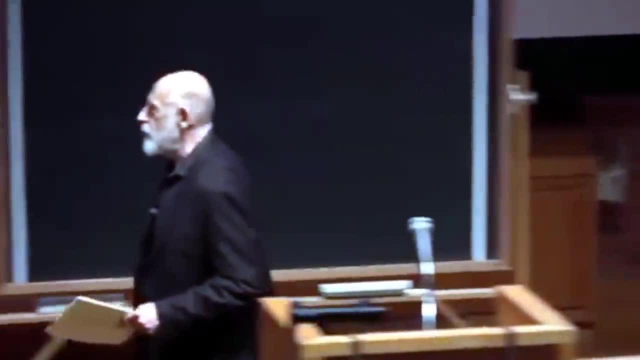 and you have absolutely no information about either of the parts of the system. Now, that's weird, if you think about it. If you think about it, I'm telling you that you have a complete description of the composite system and yet no knowledge of either of the parts. 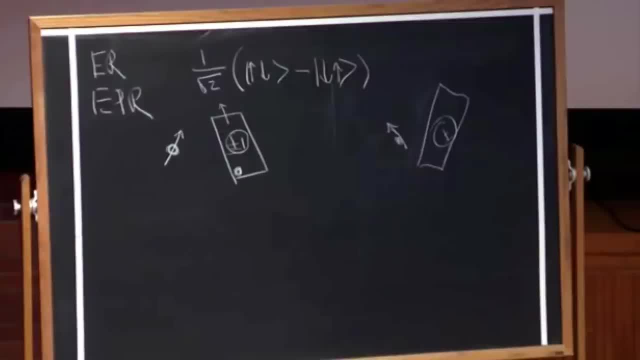 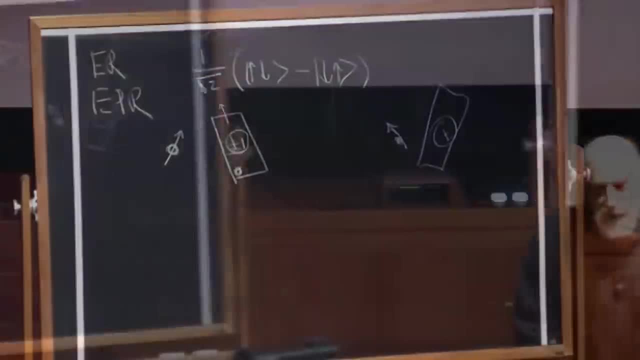 That's a feature of maximality. It's a feature of maximally entangled states. Entanglement has a degree of entanglement associated with it. We don't need to get into the mathematics of it. There can be unentangled states. there can be a little bit entangled states. 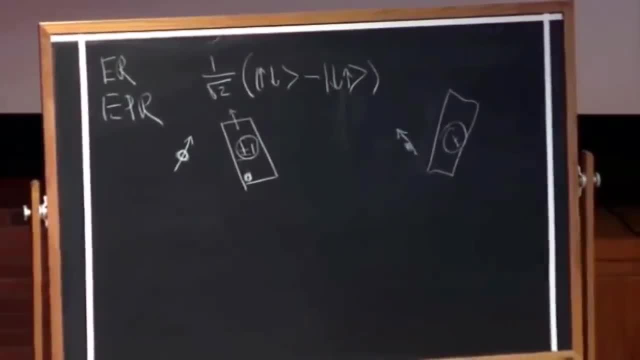 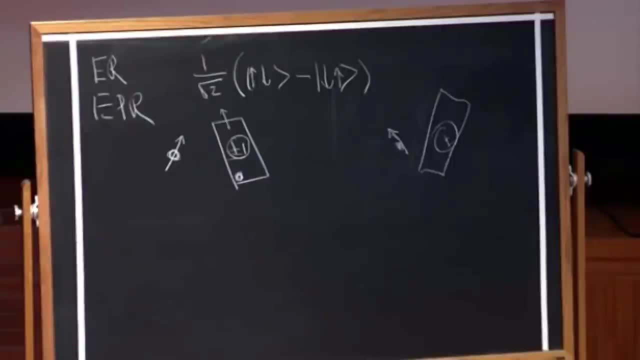 and there can be very entangled states. I'm interested in the very entangled states now. Okay. so the question then is: if everything is random, what does this thing, this state, tell you? What it tells you about is not what happens. 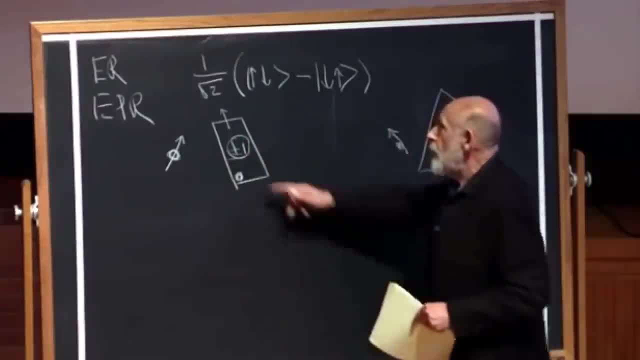 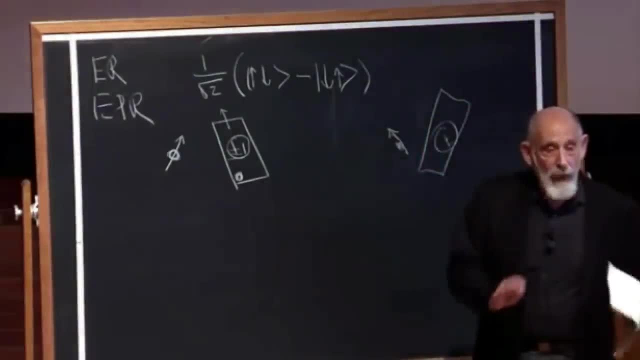 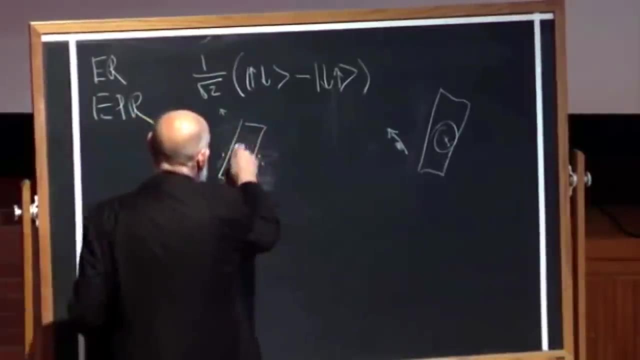 if you make a random statement like one measurement or the other one, but it tells you about correlations between the two. In this state, the following is true: Pick any direction at all. line up the two detectors or the two apparatuses in the same direction. 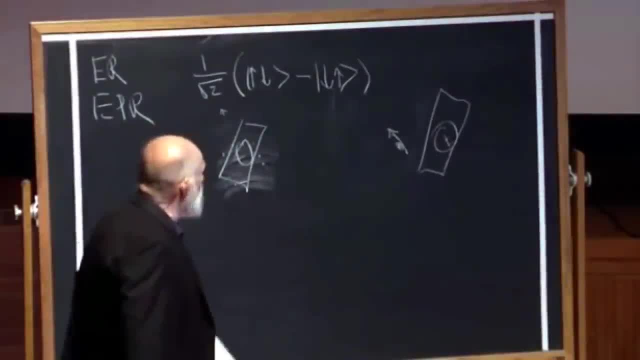 and measure both spins. In this state, here you will always- although it's random whether you get a plus or minus one- if one of them gives a plus one, the other one will always give a minus one. In other words, although the polarizations are completely undefined, 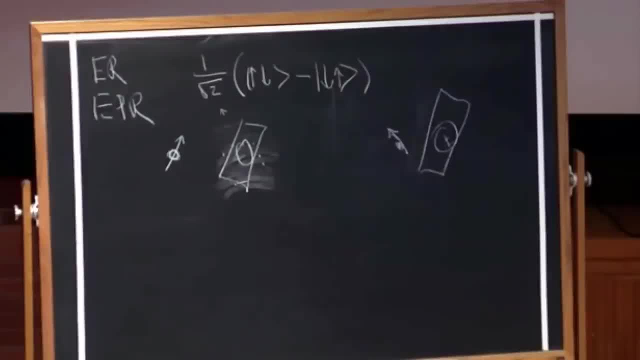 for the individual spins. nevertheless, they are found every single time to be in the opposite direction. The entanglement tells you about correlations between them, it tells you about relations between them, but it tells you nothing about the individuals That shook Einstein, That bothered him. 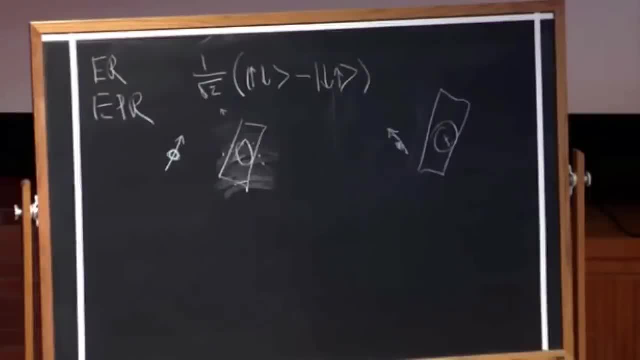 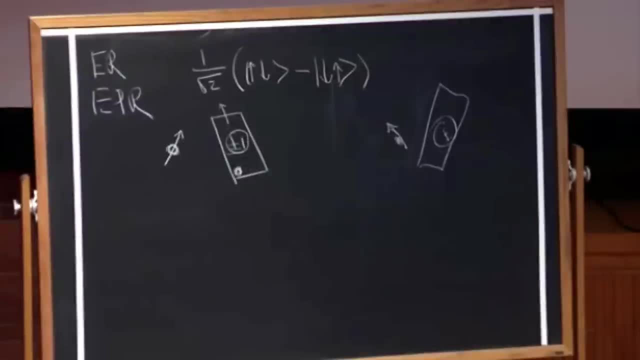 He said: what's real? What is real about these two spins? And he came to the conclusion that the description here didn't say anything about either one of them and that bothered him Somehow. Bohr just was okay with it. I don't even know if Bohr understood it. 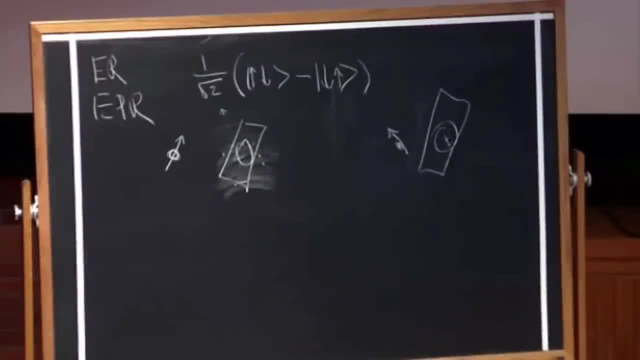 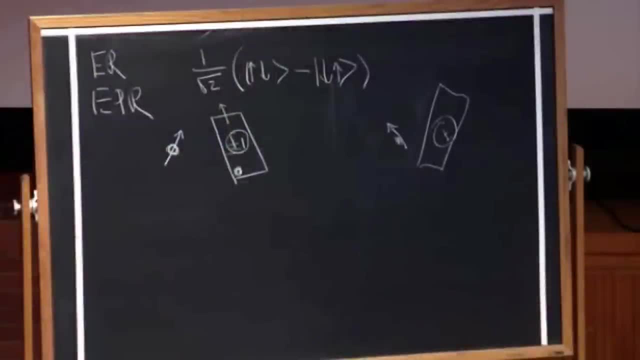 If you read the dialogue between them, you'll come to the conclusion that Bohr was mumbling in his beard. Anyway, can you simulate this system? It's kind of interesting. You can simulate it. all. right, You can simulate it on a computer or a couple of computers. 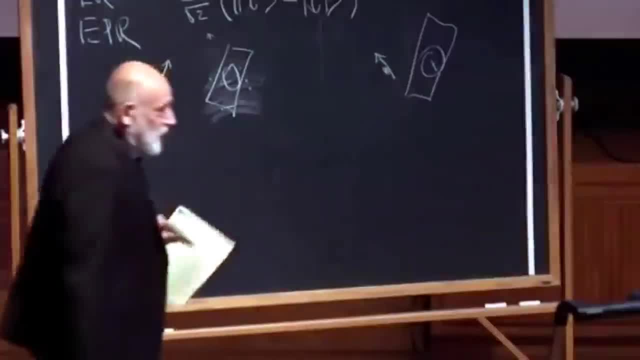 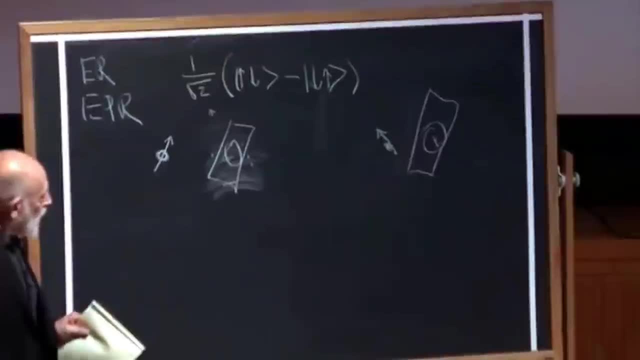 the situation of the entangle. If they're not entangled, if they're in a product state, it's easy. You just make two replicas of the detector and everything else. If they are entangled like this, in order to simulate it, you have to do the following. 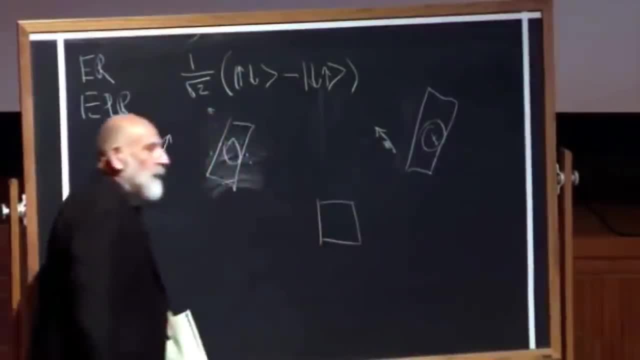 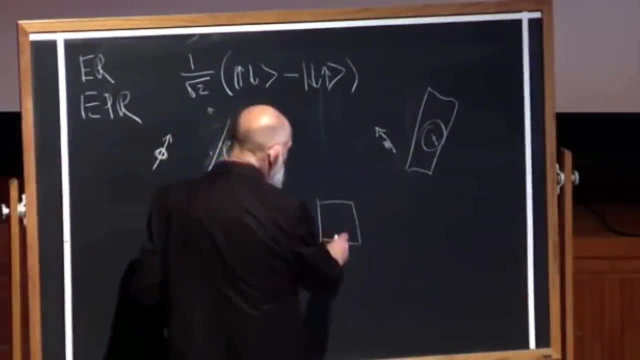 You first of all have to have a kind of central processor which is going to do the computing. So it sits in the middle there somewhere. It has to have the usual random number generator, random number generator. It has to have the usual random number generator. 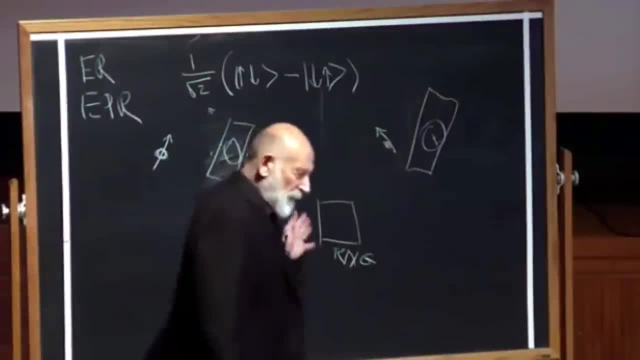 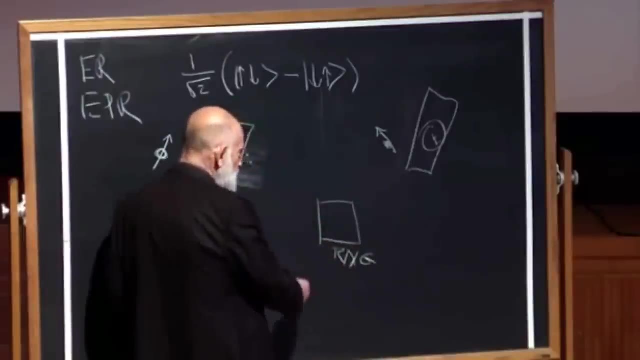 the usual memory, but now it's memorizing, not memorizing. it's remembering the state of the two-spin system, not just one spin at a time. It's remembering that state And the random number generator and associated pieces have to be connected by wires. 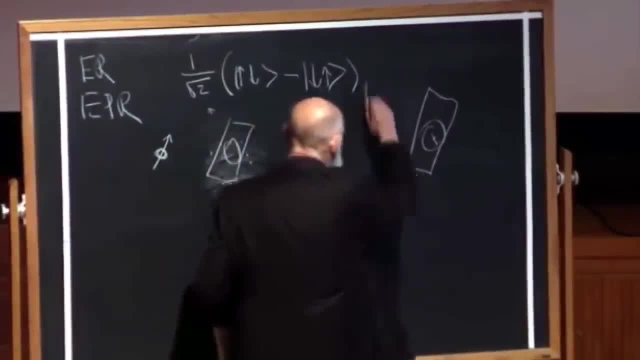 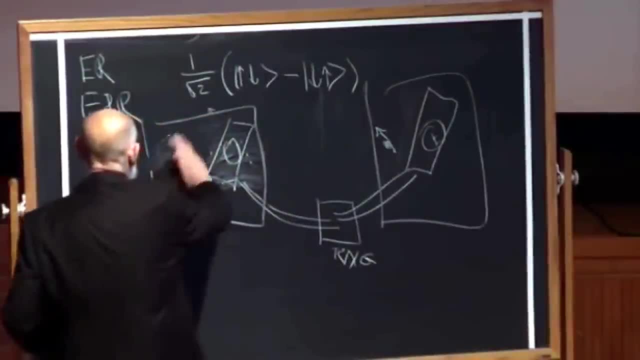 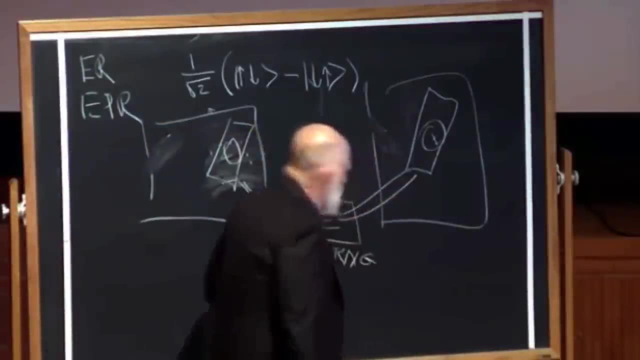 to the two distant components. So we have computers. Remember, we're now simulating it. This isn't real. There's no real electron there. There's no real electron here. We're trying to fake it. In order to fake it, there have to be wires there. 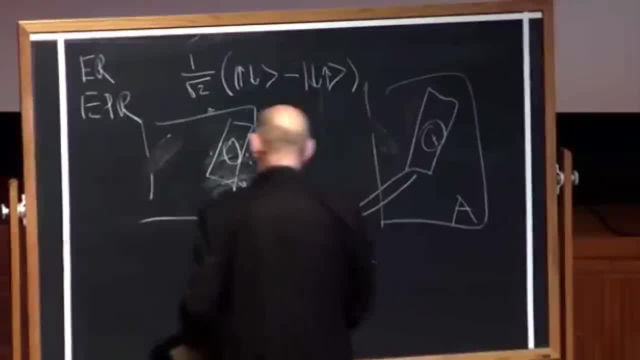 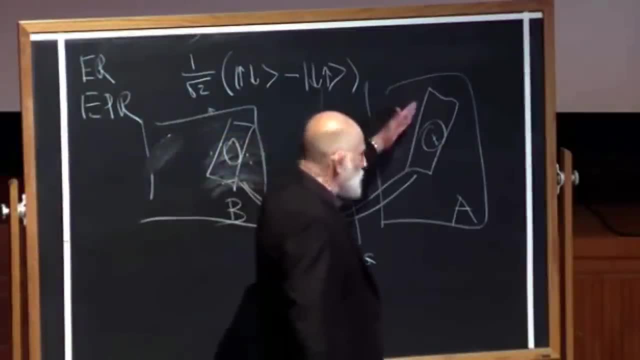 On one side. let's call this Alice's side. We'll use the usual Alice and Bob On Alice's side. Alice is going to make a decision about what direction to measure the spin in The instant that Alice decides to measure that spin. 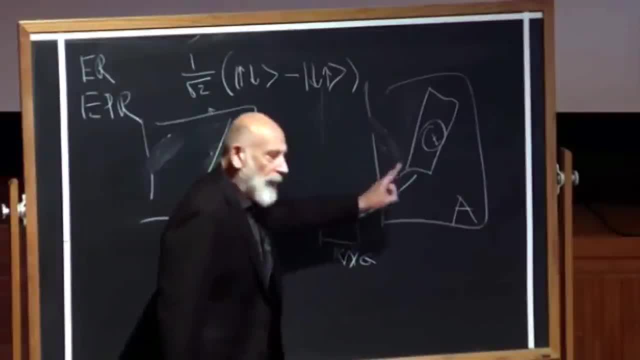 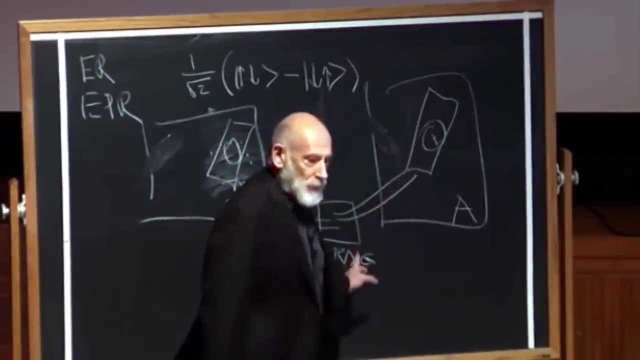 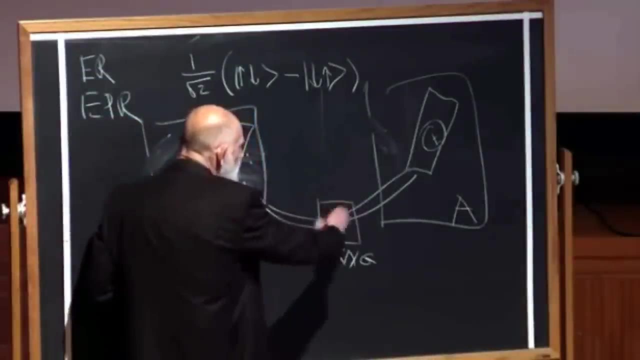 or the instant that she starts to measure that spin, a message has to go to tell the random number generator in the system over here what direction Alice decided to make the measurement, in what direction her apparatus was in. Once that happens, some things happen here. 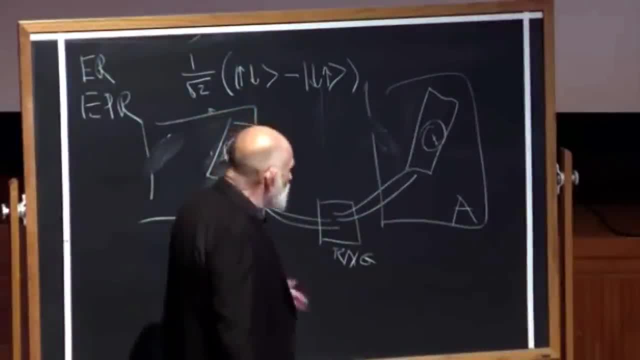 and then it sends back a message with a random plus or minus one. not a completely random plus or minus one, but a plus or minus one. that is supposed to be the answer. Same for Bob, And Bob has to be connected to the same random number generator. 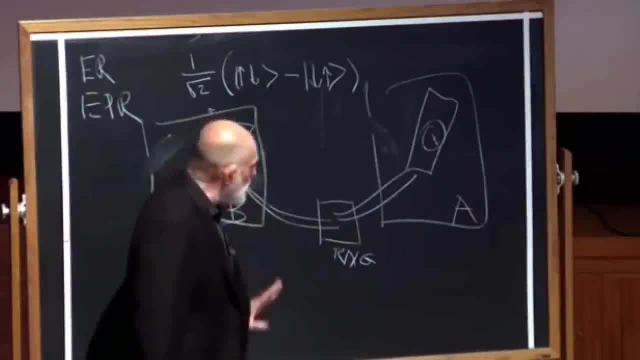 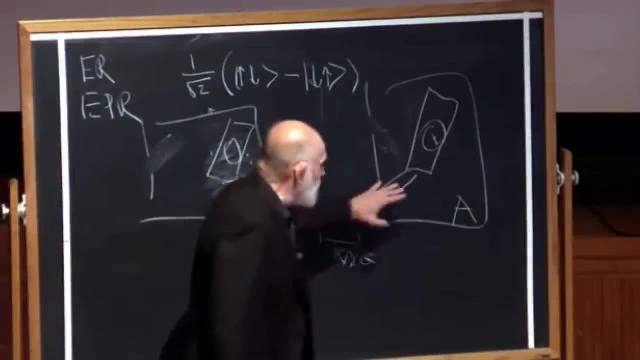 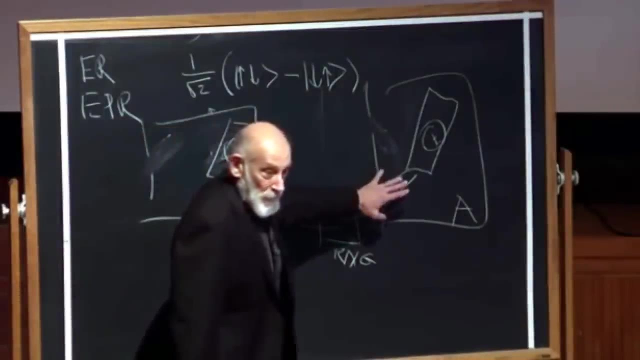 because of the strange entanglement or the strange correlation between them. So in order to mimic the quantum behavior of two distant entangled systems, you have to fake it with a collection of wires that connect them. basically, What would happen if you cut the wires? 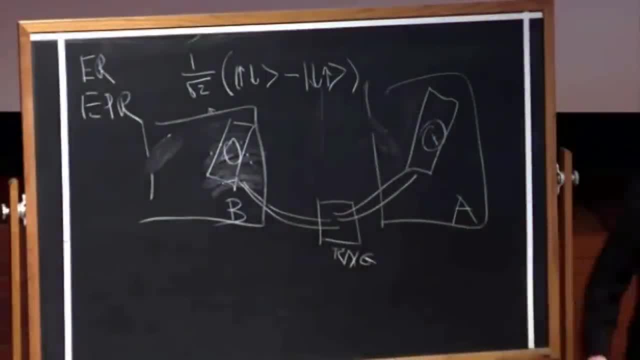 and tried to deal with it by two separate systems. You couldn't do it. This is the sense in which entanglement is non-local. It's non-local in the sense that if you try to simulate it with a classical computer, if you try to simulate quantum mechanics, 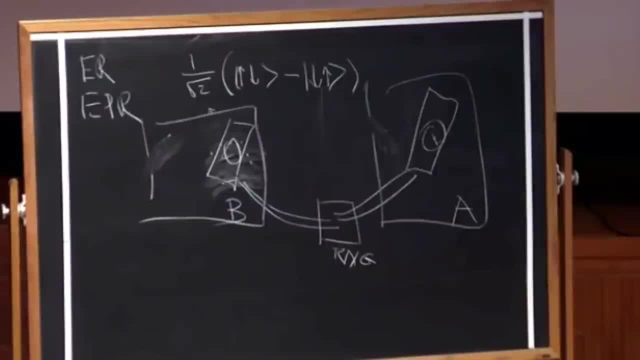 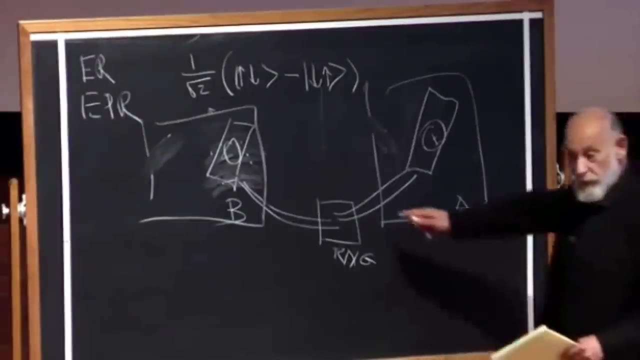 with a classical computer, you have to fill space with wires. Those wires would really have to genuinely be there and, more than that, the wires have to be able to transmit information, essentially instantaneously, to do this. That's the sense in which quantum mechanics is. 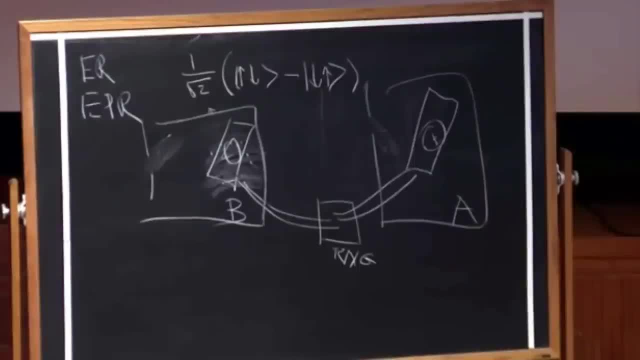 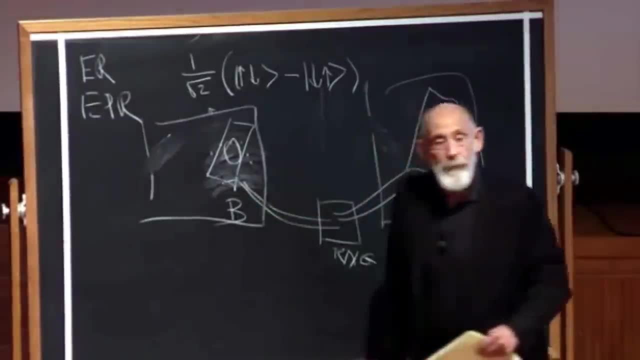 Now you may ask: with all these wires around, can you transmit information faster than the speed of light? Can you transmit from Alice to Bob a piece of information about anything you like? Well, sure you can if you have those wires there. Those wires are like telephone wires. 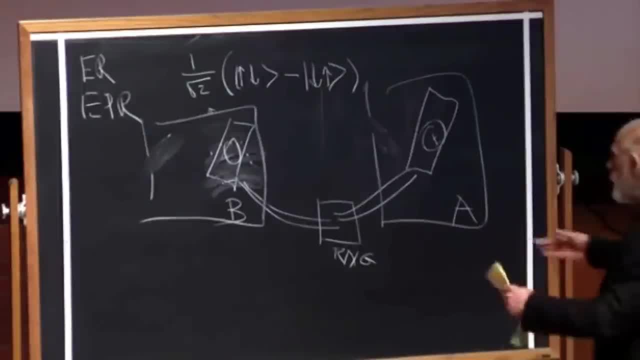 and they're instantaneous. so of course you can. So this might seem to violate Einstein's principle that you can't send information faster than the speed of light, but in fact, if you restrict yourself to only those operations which make sense for quantum mechanics, 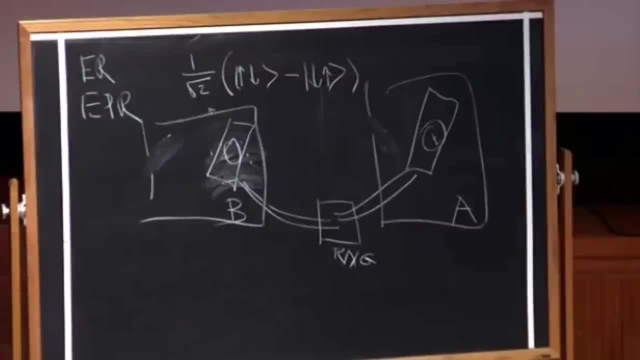 the thing that a quantum mechanics experiment would actually allow you to do. under no circumstances will you send anything faster than the speed of light. So it's a little bit strange, but the strangeness has to do with simulating quantum mechanics on a classical computer. 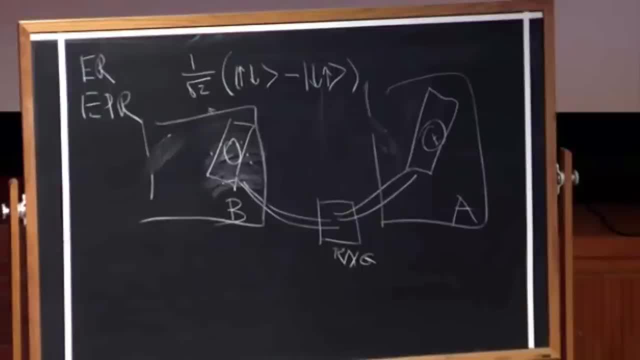 That's what entanglement is about. I'm sort of taking you through a tour of various interesting things about entanglement. Now the next thing is: is entanglement a rare phenomena? Is it something that you have to work very, very hard? 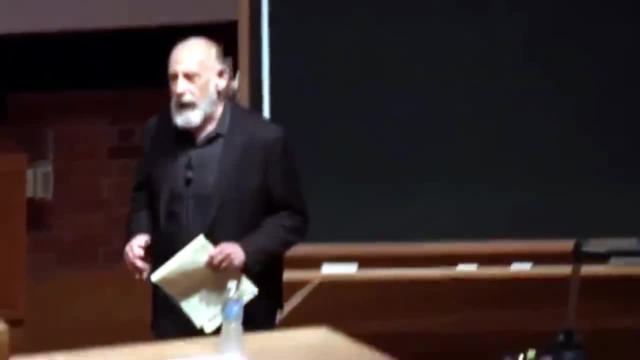 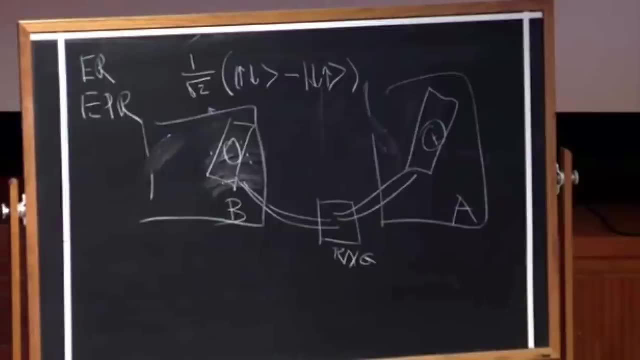 to arrange between systems. The answer is no. Entanglement is extremely generic. In fact, it tends to spread out among systems like a very badly infectious disease. If you have a system which is composed now of a lot of parts, Let's imagine we have a system. 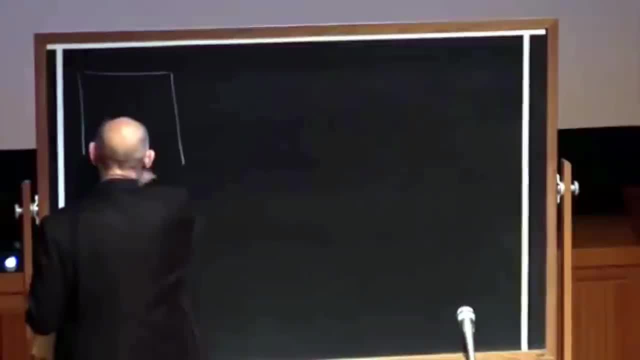 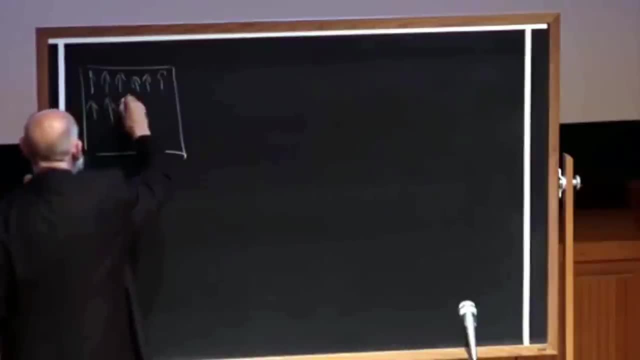 that's composed of a lot of these spins. Here it is. it's a box of spins with lots of them. Let's start them all in some particular state, which is a product state, and, let's say, in which they're all polarized. 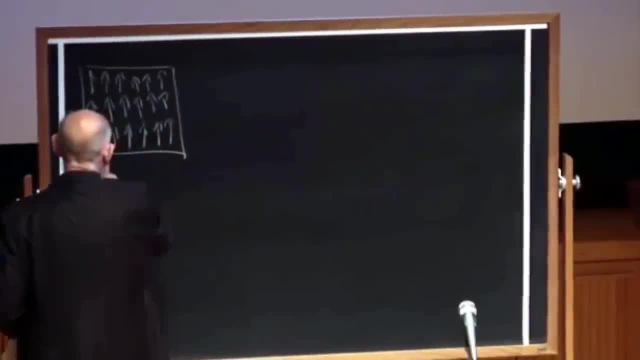 along the z-axis. I want to put some more in. I want to have an even number. Okay, We start that way. That is not an entangled state. Each one of these things is in its own private state. They are not entangled. 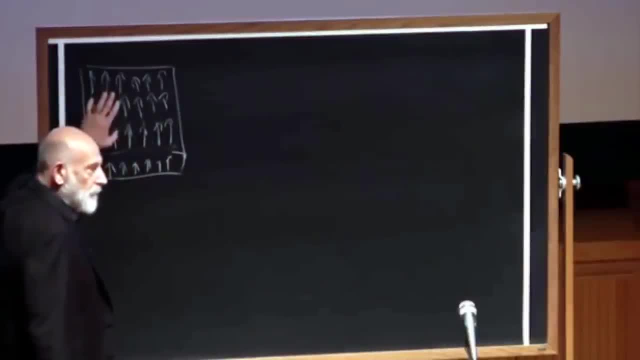 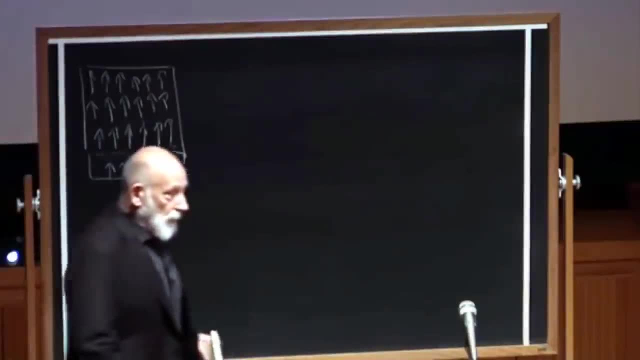 You gain no information about another one by measuring one of them, And that's not entangled. Okay, Now you let them interact with each other. You let them just interact, maybe even just a little bit, some kind of forces between them. 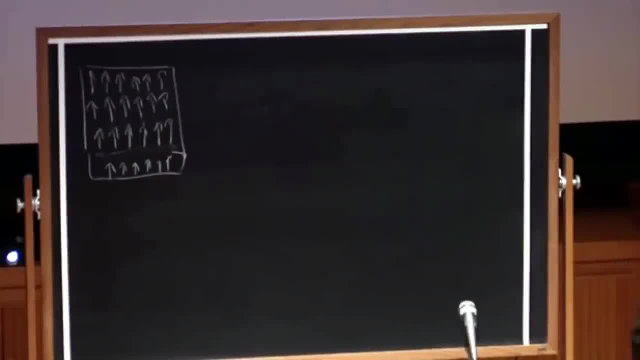 maybe some interactions which tend to rearrange them a little bit and let those interactions persist for a relatively short time, just a fraction of a second. In a very short time this system will become maximally, or very close to maximally, entangled. 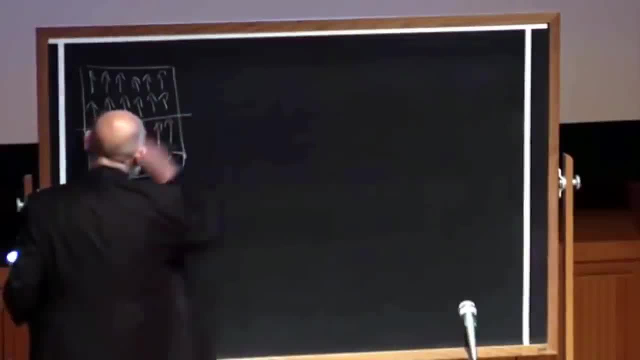 What does that mean? That means, if you divide the system in half in any way, in fact, no matter. vertically divide it in half, diagonally divide it in half, just pick out half the spins and pick out another half the spins. here's what will be true. 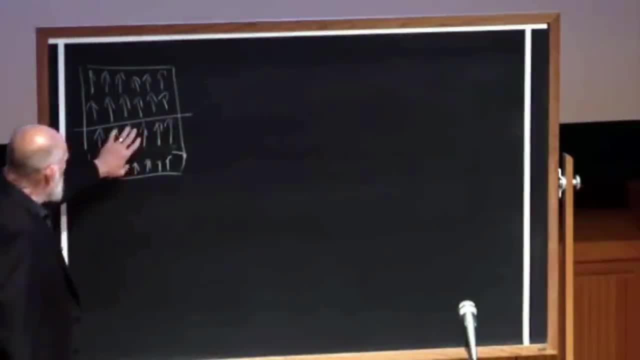 The state will give you no information about either half. Everything that you measure about either half will be completely random, But if you want to know the result of any experiment, let's call this Alice's share. let's call this Bob's share. 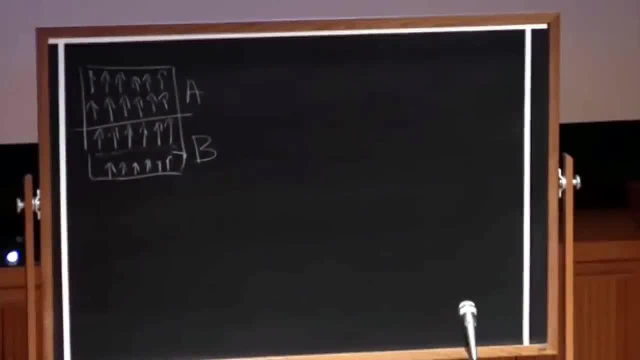 Bob can predict the result of any measurement that Alice will do by doing an appropriate experiment of his own, which will then- and it's exactly the same thing as over here- these two entangled spins. if you want to know what one of them is doing. 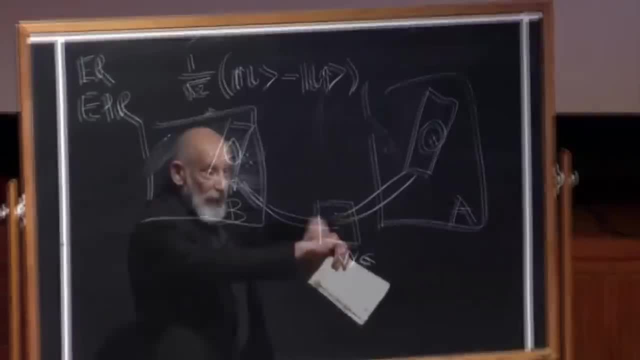 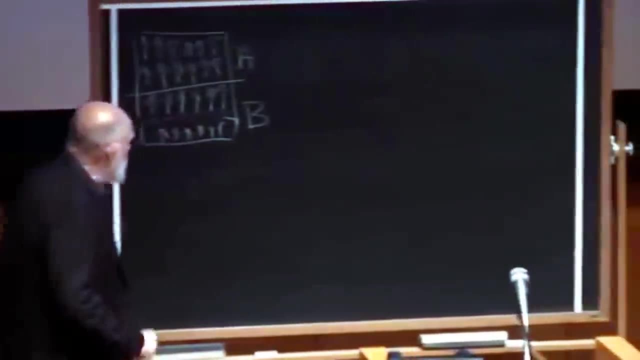 just look at the other one, and the first one will be anti-parallel with it. if you were to measure it, If you were to measure both of them, they will be anti-parallel. The same kind of thing is true here. 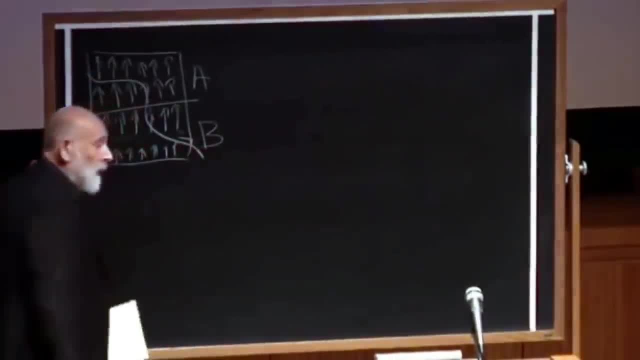 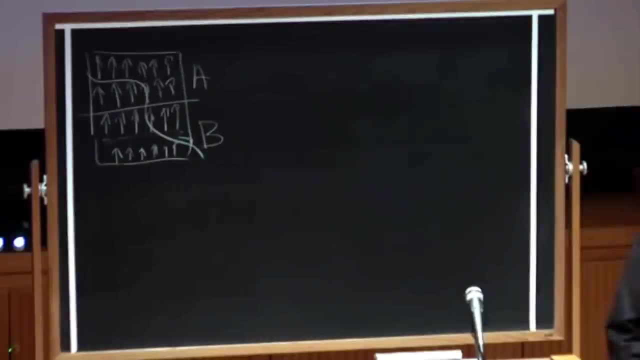 And, what's more, it doesn't even matter how you divide it. Any way that you divide it, you'll be able to predict the other half by measuring one half. That means that entanglement is very pervasive. Things tend to get massively entangled very quickly. 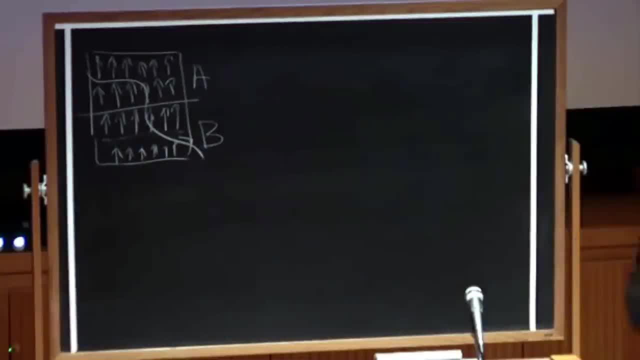 I assure you you are entangled with your neighbor. In fact, you're entangled with me. I don't know how that feels to you, but In fact you're entangled with the Martians on Mars. Okay, Let me give you another example of entanglement. 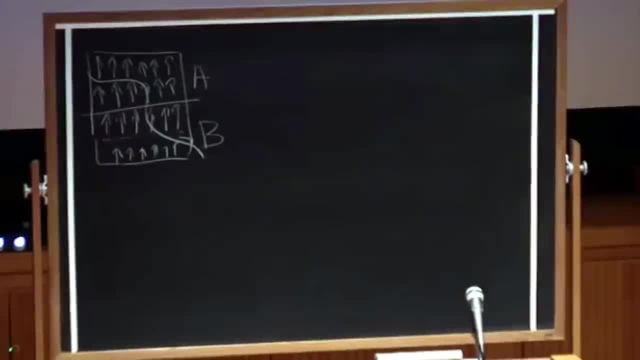 In this case, it's not entanglement of spins, it's entanglement of regions of space. It also makes sense to talk about entanglement of regions of space. So here's two regions of space And let's say the question that we can ask. 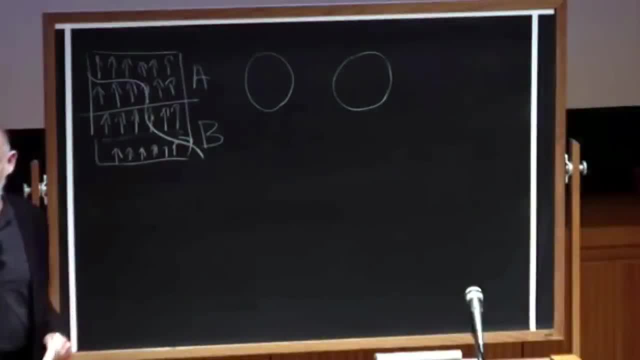 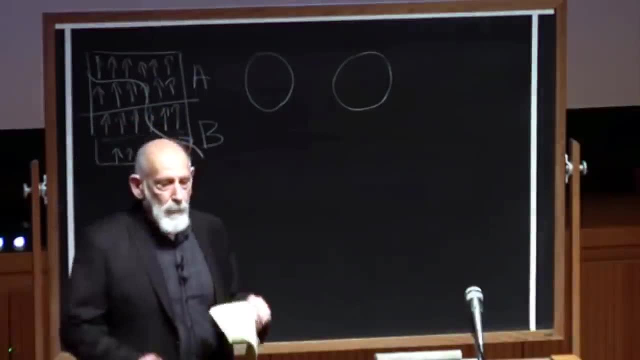 about these two regions of space is: is there a particle in there or not? Is there a particle in here? Is there a particle in here? Okay, One possible state of the system is what you would call a product state In a product state.